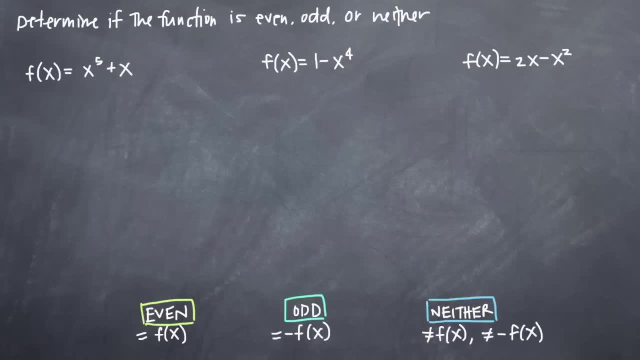 function or neither. To make this determination in each case, we'll plug in negative x in place of x to our functions. simplify and then the result will tell us whether the function is even, odd or neither even or odd. Let's go ahead first and plug in negative x to our 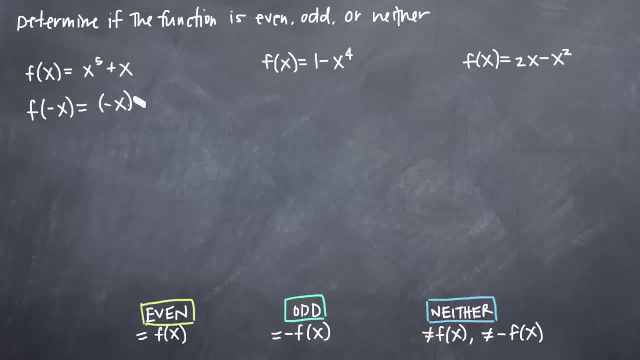 first function. We'll get negative x to the fifth plus negative x to the fourth. Again, we just want to simplify as much as we can here. Negative x to the fifth will give us negative x to the fifth like this, minus x. At first glance this might not look. 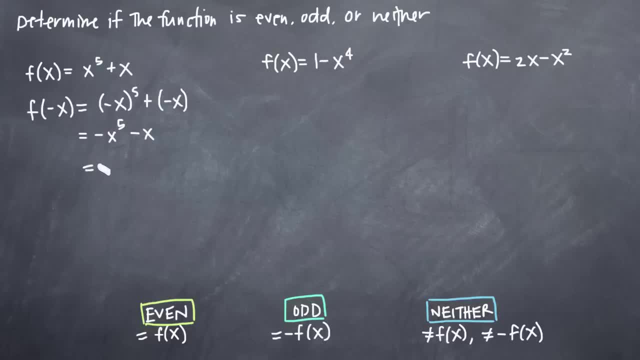 the same as our original function f, but if we factor out a negative sign we'll get negative x to the fifth plus x. We can see that our functions are the same but for the negative sign out in front We have in our original function x to the fifth plus x and in our simplified function. 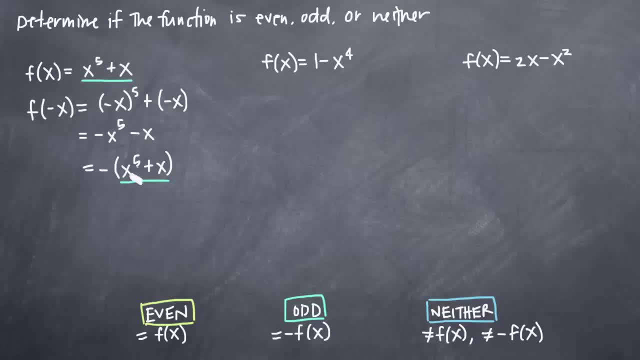 here x to the fifth plus x. the only difference here is this negative sign. As you can see, since we know that f is equal to x to the fifth plus x, we could just as easily substitute f for x to the fifth plus x and you can see that we get negative f. That's exactly. what we were looking for. To determine that this is an odd function. we're going to need to find the negative sign. We have to find the negative sign and we're going to need to find the negative sign. and we're going to need to find the negative sign. We're going to. 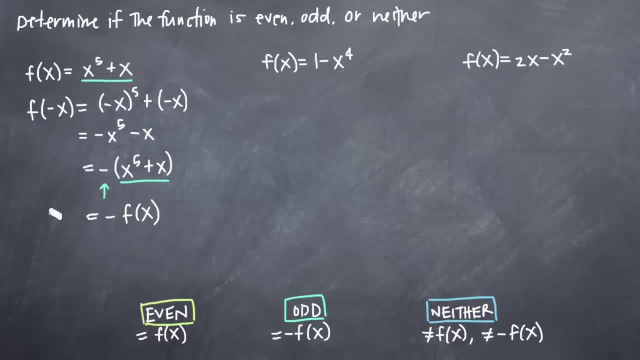 find the negative sign. so we know here that we have an odd function. We'll go ahead and do the same thing with our second function. As always, we're going to plug in negative x in place of x and we'll get 1 minus negative x to the fourth When. 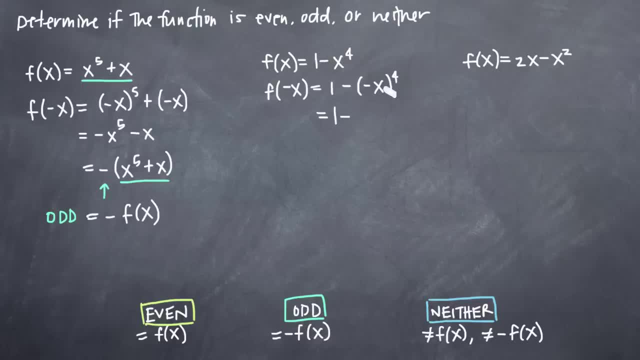 we simplify this, we'll get 1 minusnegative x to the fourth will give us a positive sign. that negative sign inside the parentheses will go away and we'll just be left with x to the fourth, back where we started, at f of x. So this just becomes f of x and, as you know, when we get 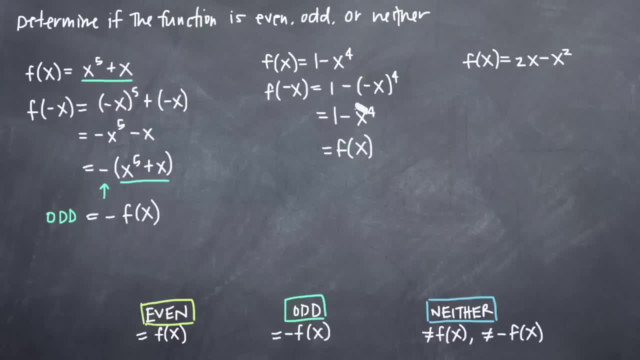 back to our original function, f of x. we know that that's an even function. We've defined these down below. by the way, We can see that if we get back to f of x, we have an even function. If we get to negative f of x, as we did in the previous problem, we have an.